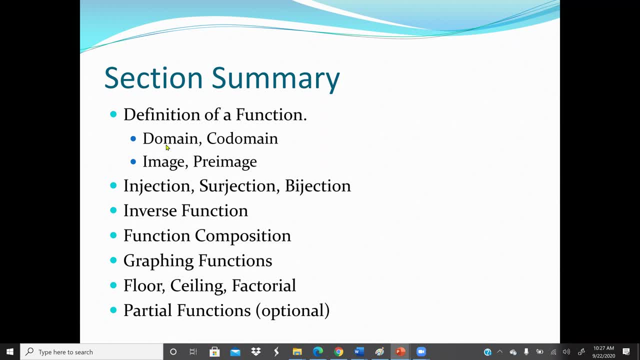 function and we're going to study some field terminology. what is a domain, co-domain, image and pre-image. Also, what is injection, subjection, bijection, Also inverse function, function composition, graphing functions, floor ceiling and factorial and also partial functions. 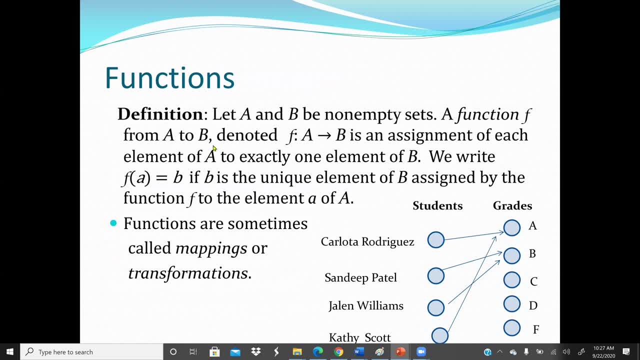 So first we start with the definition of a function. Here we select A and B, B non-empty set. So a and b are set with some elements. So a function f from a to b will be donated as a in pride to b, And here we say it's an assignment of each element of a to exactly. 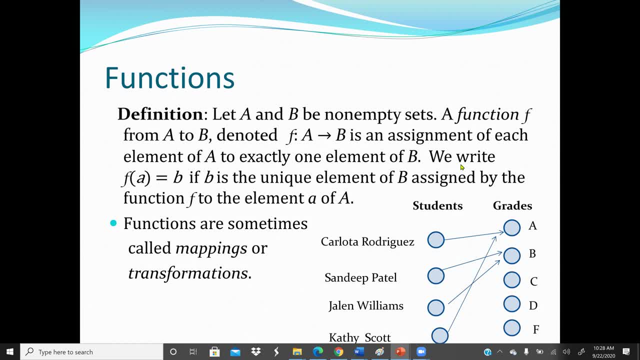 one element of b and we write f at equal to b. again, if b is a unique element of the b set, The uppercase b is the set assigned by the function f to the element a of set a. So again, what this definition means is that always a function may have an input and output. 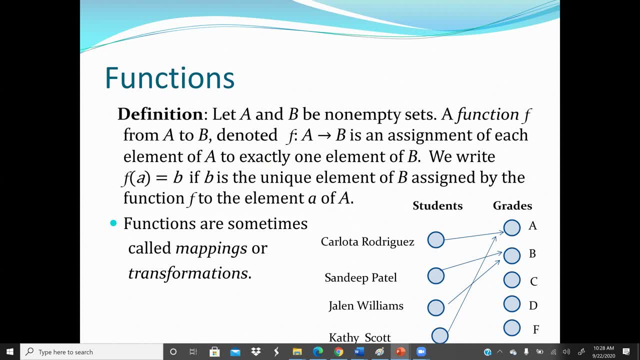 or dependent variable, independent variable. So let's assume that A is our input variable and B is our output. In college algebra we may say a function, f at x equal to y. x is the input variable, then y is our output. Now, in order to have a function, the input, 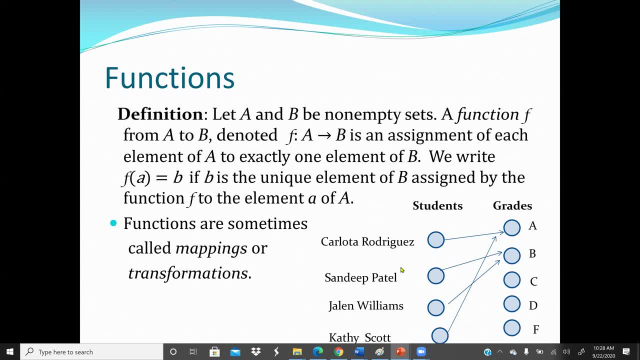 variable must generate only a unique output variable. So an example here is: if I have a student, let's say a student named Rodriguez, So here we have a function at student equal to grades. So the student will determine his grade based on how he prepared for the exams. 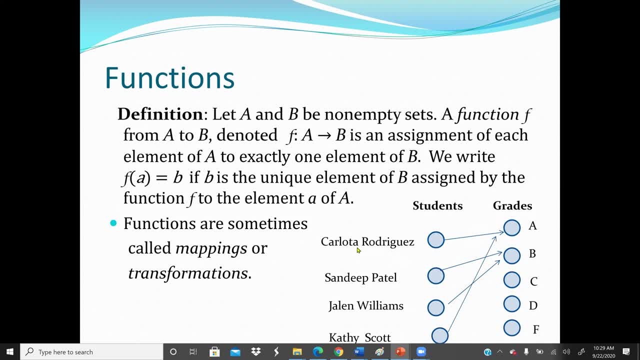 and he took the exams. So here, if Rodriguez is a student generate a grade of A and all of the students generate only one unique output, or even two students can generate the same grade, then it's a function. But if we have 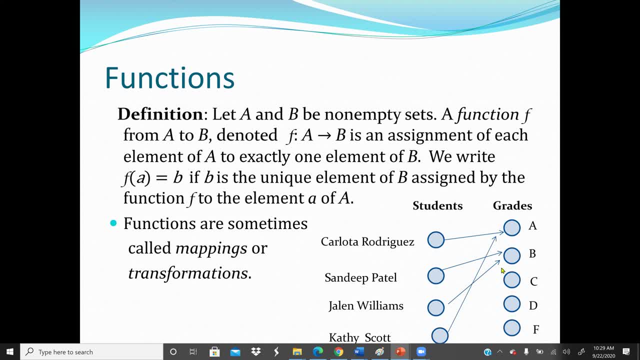 Rodriguez, that generates A and also generates B, then it's not a function. So normally in college algebra we use a vertical line to check if it's a function. Okay, a�, 좋아하는 tu'sks 않고. Snap д queen. 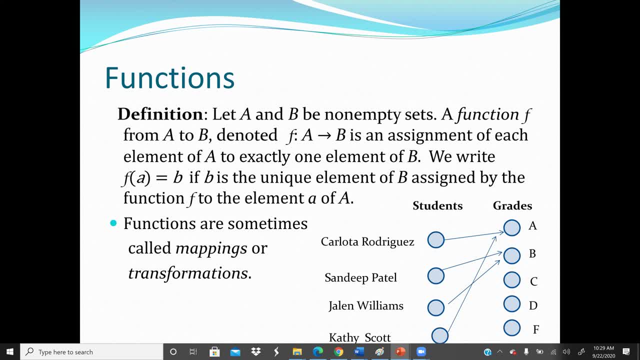 Well, for example, looking at the graph, we are going toяти acマn X간. we draw a vertical line to a function anywhere. it's a function anywhere, at any X value of A. Now, if the vertical line can produce two points on the function, the, the function is gone. That means we can have 1. 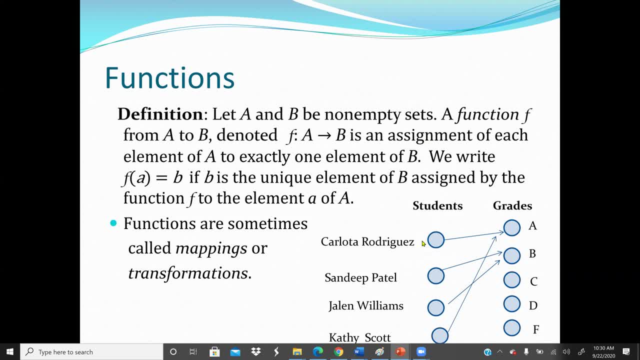 input A, x and we can generate two outputs. That means we have 1 input and we can generate two outputs. In other words, Bowser can generate Felbashed to do that. That's one way of understanding output. So our S will be the horizontal. I draw a vertical line, which means S is constant. 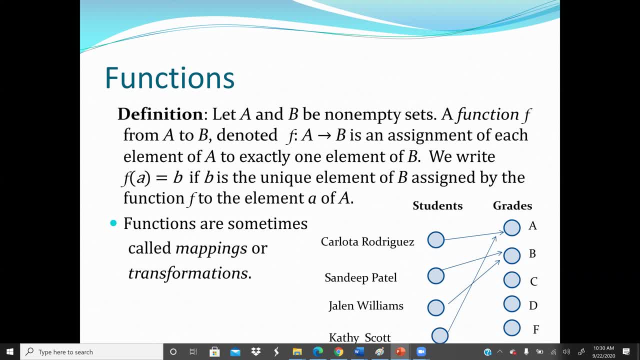 on a- sorry, I draw a vertical line which means S is constant, But Y can be any value. Now if we have two values of Y, the intersection on the graph, with only one S value, then it's not a function. So that's what we mean by this definition Here we are trying to 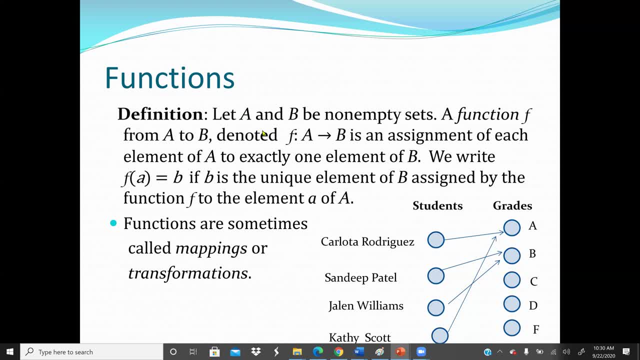 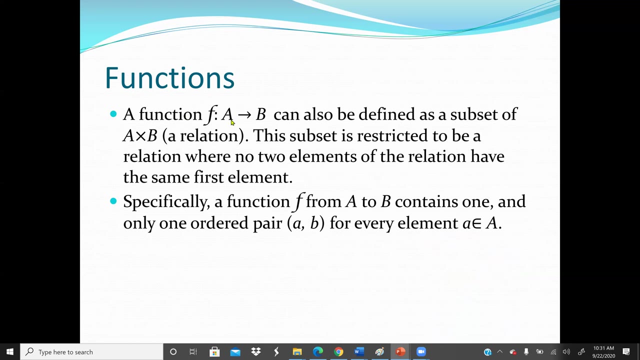 say that the set A element can only generate set B element uniquely. One element will generate one set A element will generate one set B element, which is the output. So again you have a function with a set A in price to B can also be defined as a subset of A by 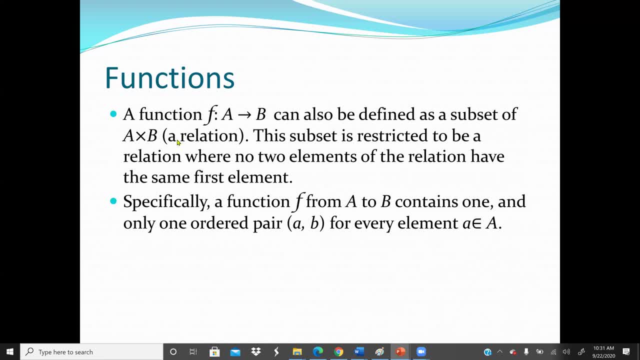 A, B. that's the relation of the elements. this subset is restricted to be a relation where no two elements of the simulation have the same element, first element. so this is what we mean. again, there's no way that we're going to have an input. let's say here, I want put to be the element of a. there's no, any element. 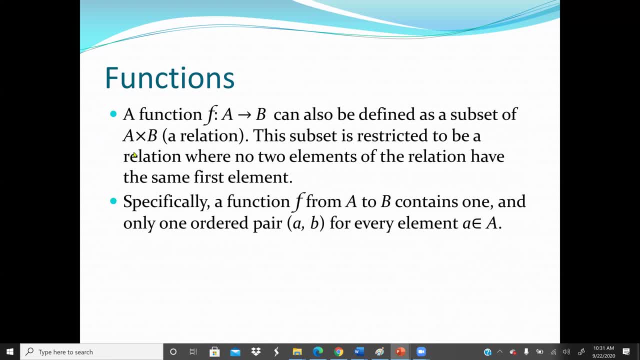 is set a that can generate two output, that's a: two element in set B. that means it's not a function. if an element in set age generate two or more element in B, it's not a function. so a function means element in a. we generate only one. 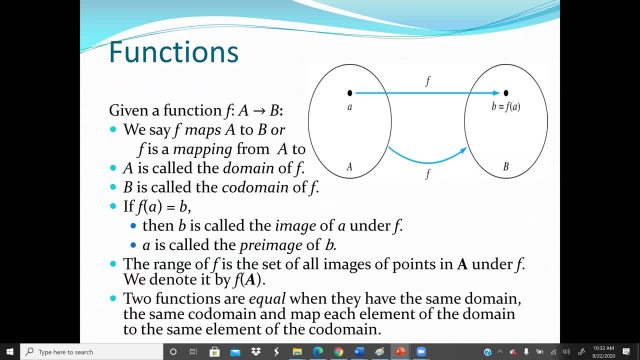 element in B. this is the example from the diagram. so we have a, a, a lowercase a in a set of a case a, element B in a set of a case B. so a, we generate only B and we say here the function is moving from A to B, right? 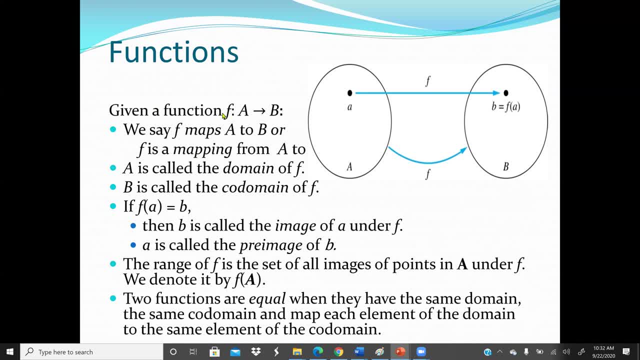 here. then here we have a function. so give you a function: F in in a set of values available in this set: A, B, F, A and F in the set of values in this set: A, B, F, B and F in the set of values available in this set: A, B. we can: 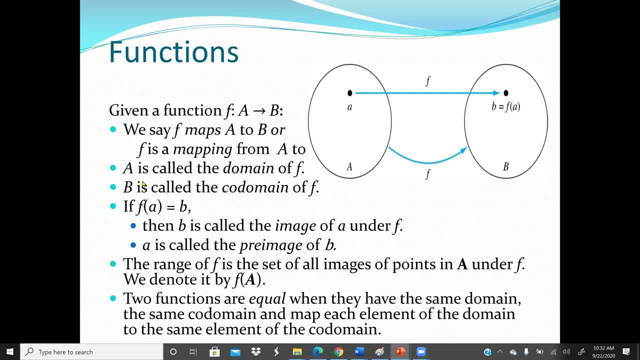 say F maps to A to B or F is mapping from A to B, A will be called the domain of the function. so our input to be the domain of the function and the B is called the Codomain of the function. in college sometimes the B also is called 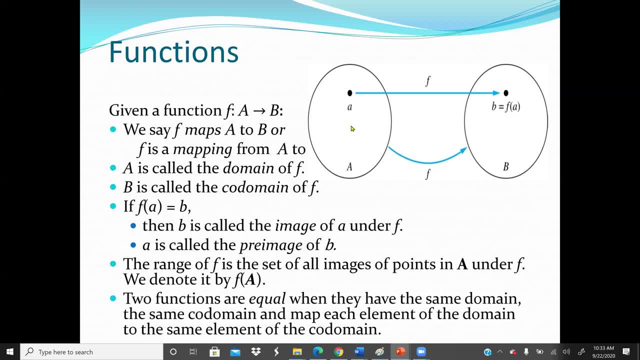 the range, so A will be the set of input variables, then the B will be the range of. Then we can also say that B is called the image of A under F, So B is called the image of A under F, And A will be called again the pre-image of B, So A is called the pre-image. 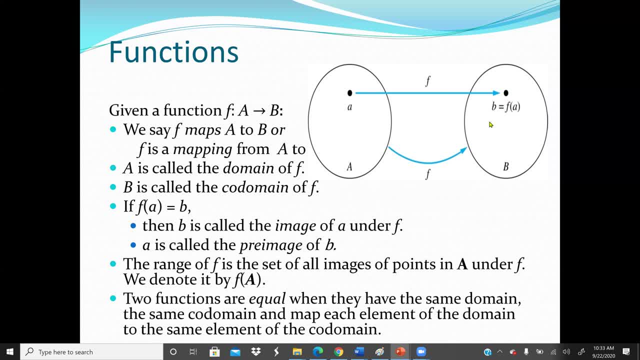 of B, Because A will generate the pain. Then the range of the function is the set of all possible images of point A under the function And we can denote that by F at A. So F at A, we start with the element. Any value we generate from F at A, B, C in the set A element. 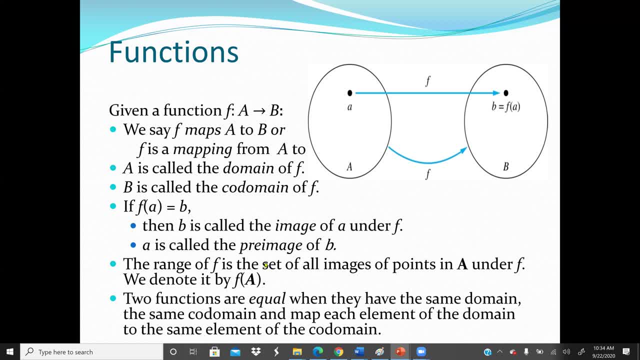 in set A Will be called again the range or the co-domain. So here also we say: two functions are equal when they have the same domain. And not only that the same domain, but they also generate the same range or the same co-domain. So two functions are equal when they have the same. 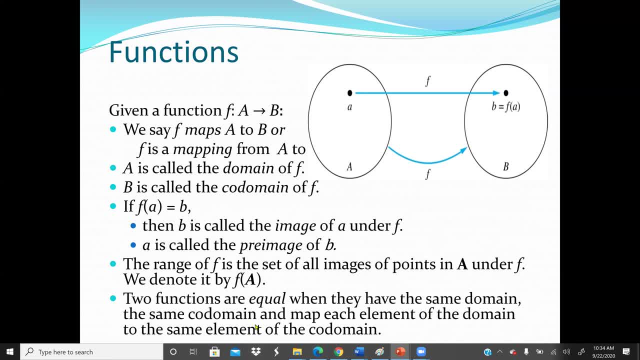 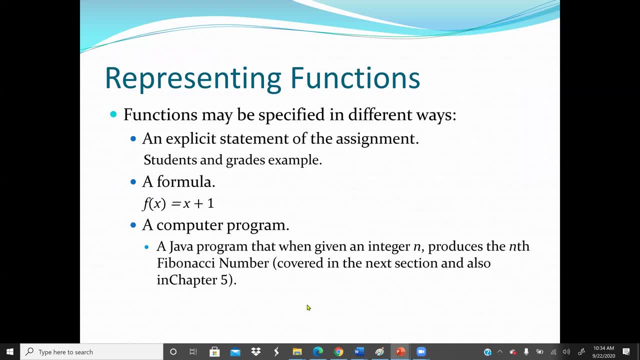 domain and the same co-domain and map each element of the domain to the same element of the co-domain. Okay, So representing a function, here we say the function may be specified in different ways. It can be an explicit statement of the assignment, Example: students and grade example, Or we: 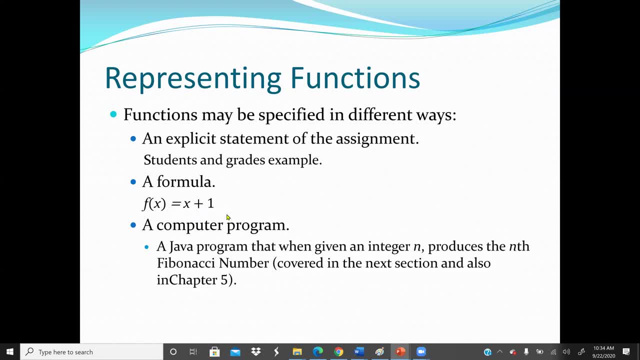 can have it as a formula F at S equal to S plus one, Or as a computer program. So function can be represented in three ways here: An explicit statement of the assignment, Students and grade example, Or a formula F at S equal to S plus one, Or a formula F at S equal to 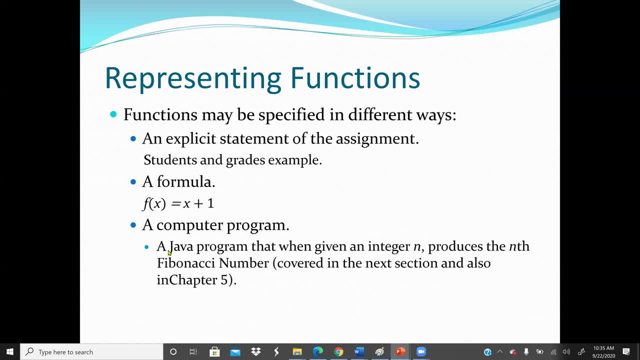 S plus one, Or a formula F at S equal to S plus one, Or a computer program- Here we say a Java program- that when given an integer n we produce the nth Fibonacci. So our function name is the function that will give us the Fibonacci of a number. This will be covered. 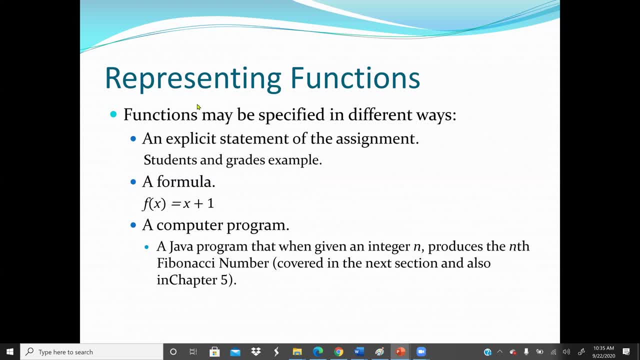 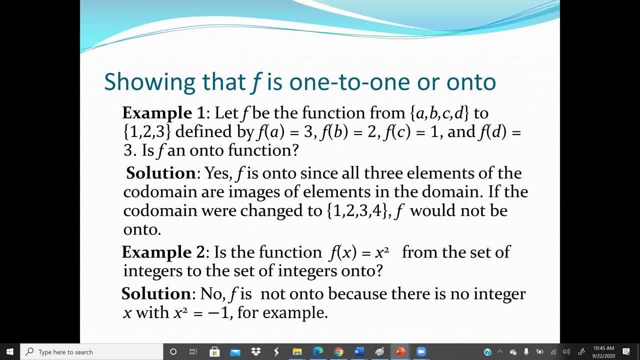 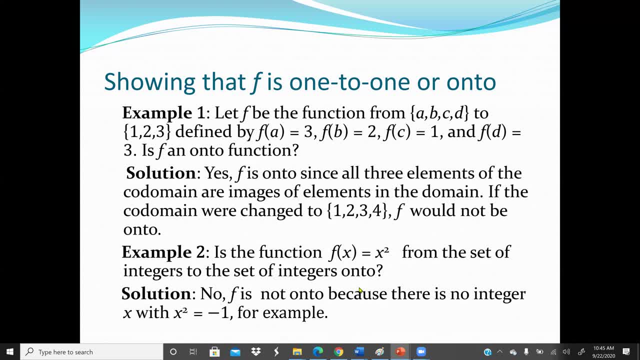 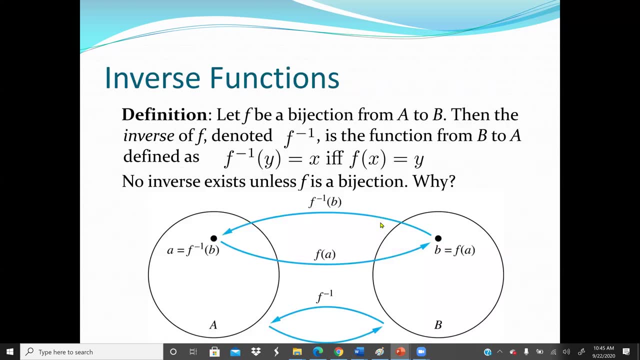 the, The, The, the, The, the one to one or on two, because on two means every input will generate the output. we also have inverse functions. the inverse function, the whole concept, is that we change the input to output, output to input. so, if I have f at s equal to y, 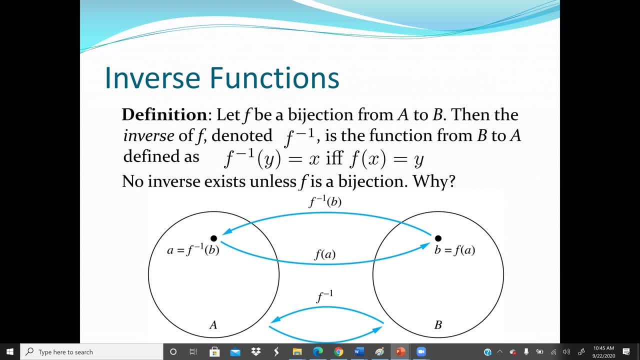 the inverse of f at s equal to y, will be y raised to the power one, I mean f raised to the power negative one, then at y. so the x will be substituted with y and again f will raise to the power negative one, which represents the inverse of the function. 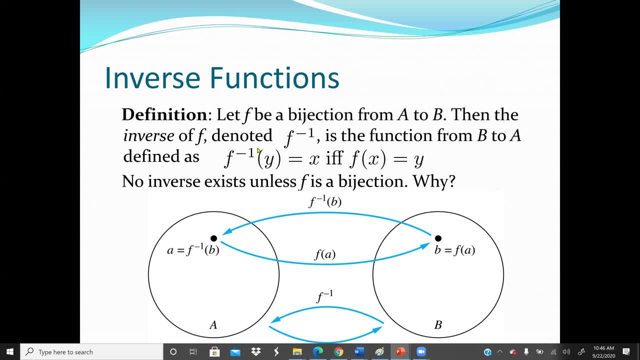 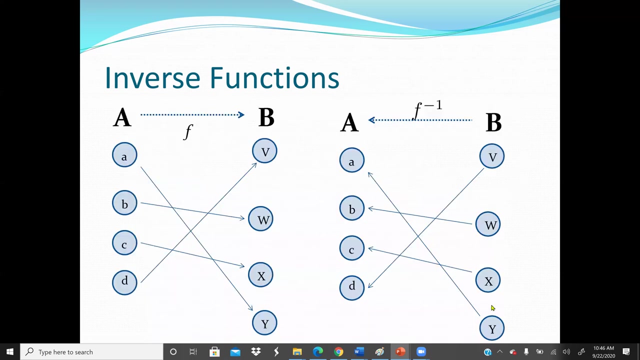 so again here we select f by injection from a to b, then inverse of f, donated by f to the power, negative one is the function from b to a. normally the function is a to b, so inverse will reverse it from b to a. so this is our inverse functions. 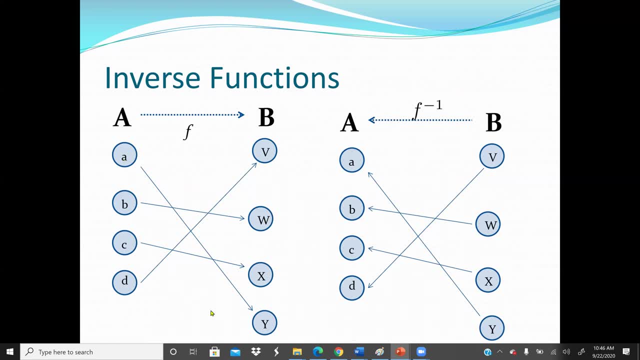 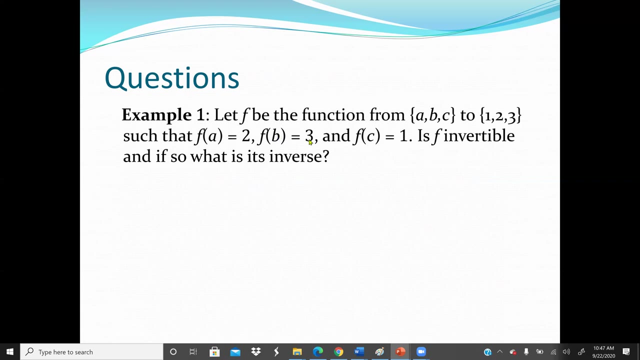 so previously we have a to y, now it will be y to a. the arrow direction changes. now we have a function question here saying that let f be the function from a, b, c to one to three, such that f at a equal to two, f at b equal to three, f at c equal to one, is f invertible, and if so, what is this inverse? 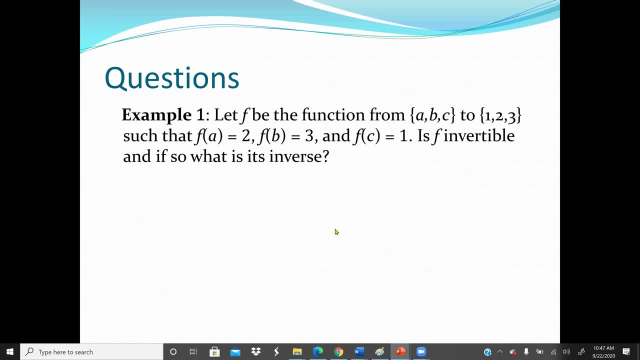 so we want to know if the function is in inverse. so what we're going to do is that we say the function is invertible because it is one to one. the inverse function. reverse the corresponding given by f. so the inverse of one is c. the inverse of two function is a, the inverse of three is b. 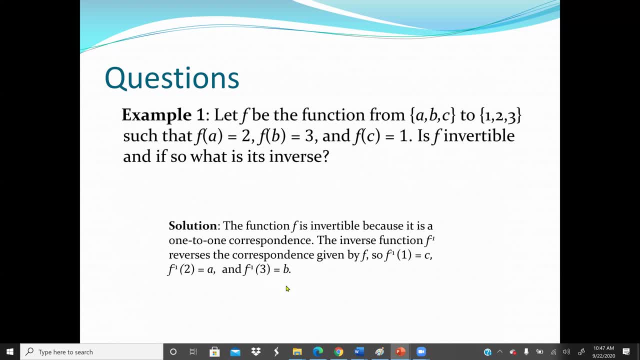 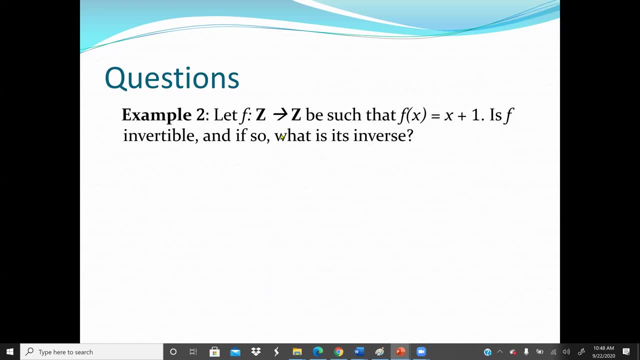 so example two: we have a f at x equal to s plus one. now, if f is invertible? and if so, what is the inverse? so we have a function f at x equal to x plus one. want to find the inverse of it. so the function f is invertible because it is one to one corresponding. 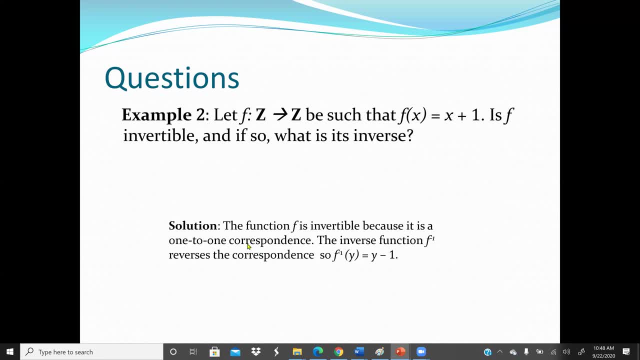 so the inverse again will not work here, sorry. and the function f is invertible because it is one to one, s plus one. so the inverse of this function, f at y equal to y minus one, will invert the positive to negative, f at x equal to x square. this will be not invertible. as we said earlier, there will be. 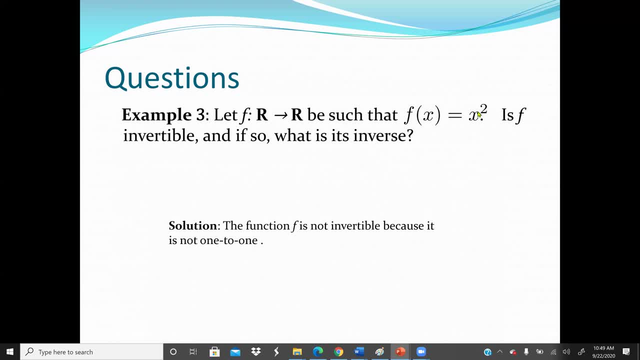 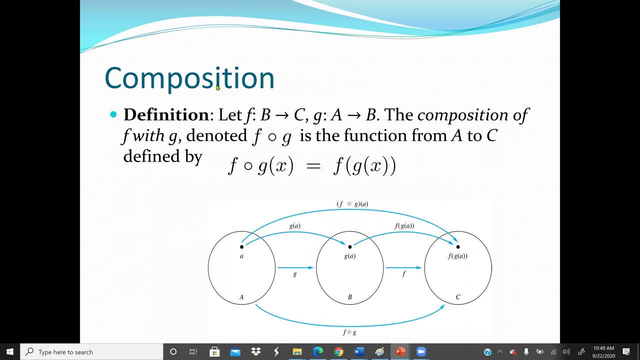 negative values, but with this function square, the values will be positive for always. so so so the function f at x equals to r square is not invertible because it's not one to one function. we also have a composition function. a composition function is a function that is: 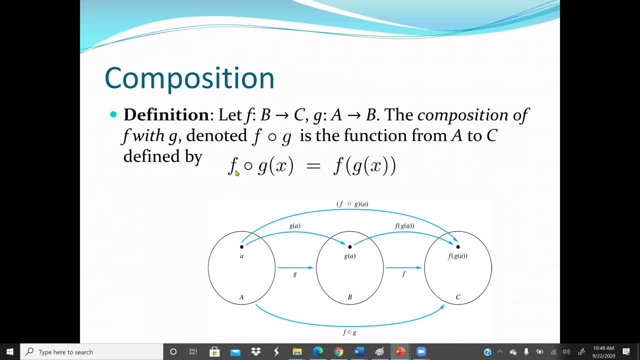 insert another function. so, for example, if we have a function f and g, the composition function f at g at s square. this means g at s is outside and it's inside the function of f at x. so you know where we see s. we replace it to the. 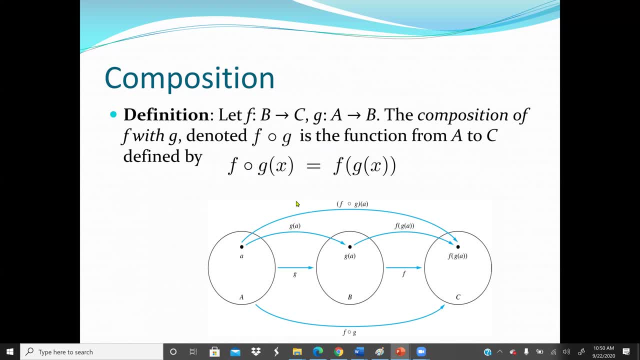 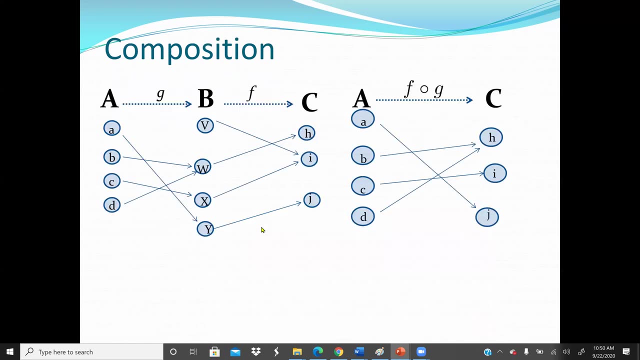 again the function name, so we see an example soon. so for example this time for f, composition, g at x, or we can write it f, g at x, and here we have the functions with elements a's, then function b and then c, so we can see that g go from a to b. 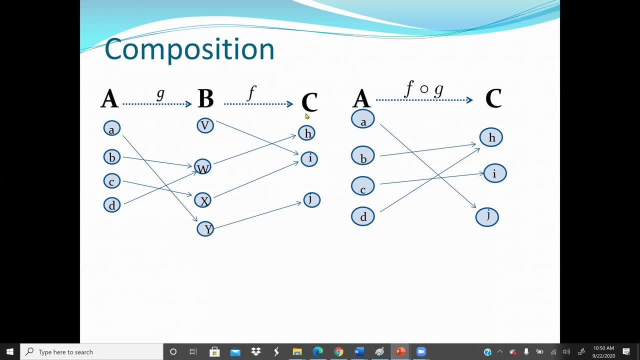 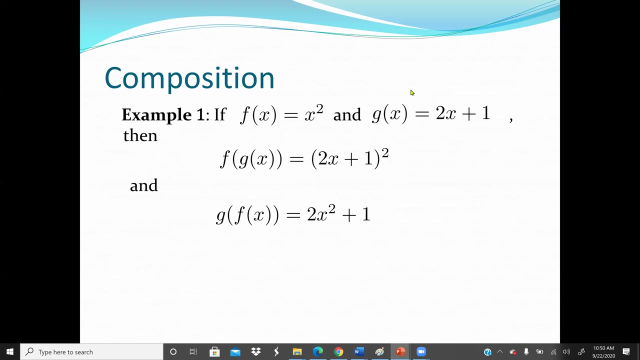 then f is from a to c. when we combine as a composite we may have from a to c now. so it will be f composite g. so here we have two function f at s equal to l square, g at s equal to two s plus one. now to find f, g at s, or we: 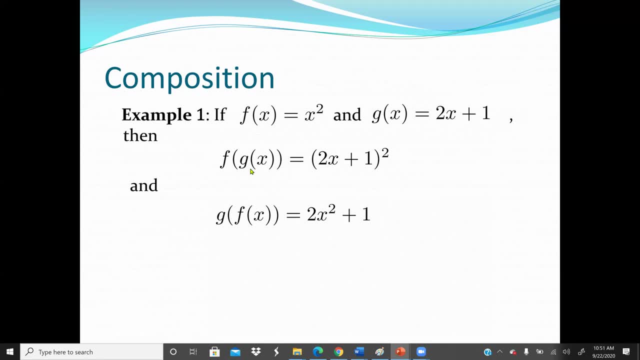 say f composite g at s. it means i'm going to write down the function f at s, then the variable x anywhere, c, x. i'm going to replace it to the second function, which in this case is again two s plus one. so here it's only x squared. so we. 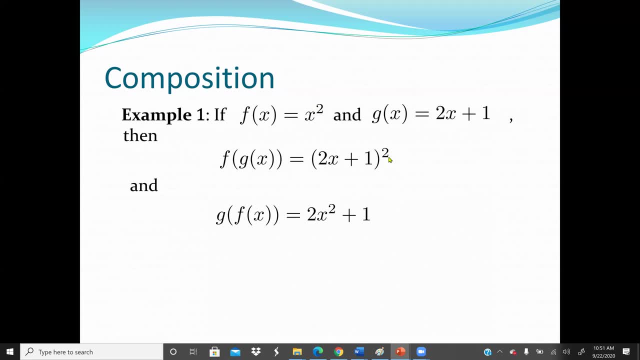 replace x, we get two s plus one by square, so we square it. now. if i'm going to find g, f at x, first i'm going to write a g, then anywhere c, x, i'm going to replace it with a square. so we get two s squared plus one. 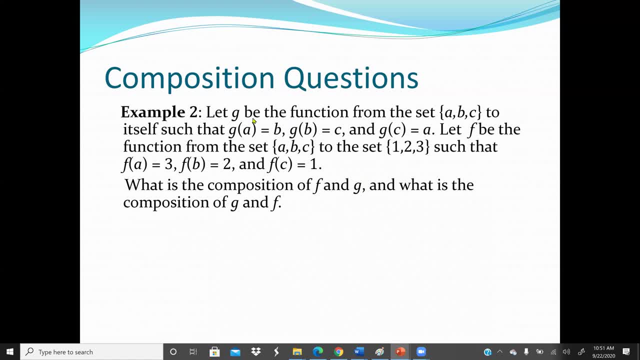 so you have another example. you're saying: let g be the function from the set a, b, c to isf search. search that g at a equal to b, g at b equal to c, g at c equal to a. now let f be the function from the set a, b, c to the set one, two, three, such that f at a equal to. 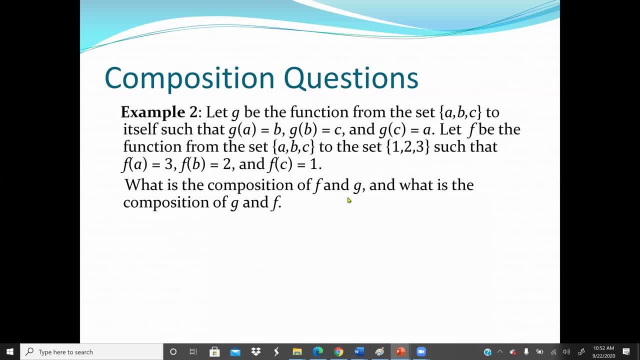 three: f at b, equal to two. f at c, equal to one. now we say: what is the composition of f and g and what is the composition of g and f? so first let's try f and g. f and g will work because we know f and g means anywhere. we see g, we are going to substitute f. 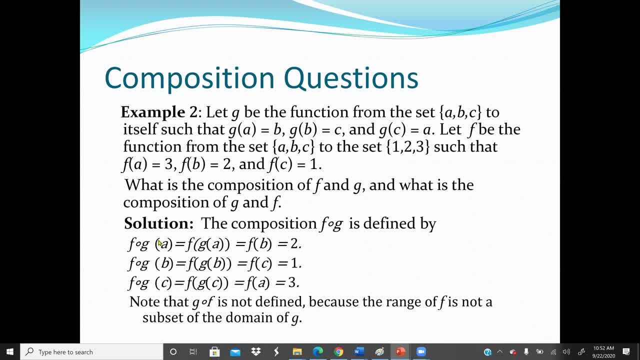 because it's f g, so anywhere g. so in this case we look at a, g at a, g at sb. so we get, give that b to f and b, which is p, so the answer will be b. so f composite g at a, equal to f g at a, and it will be f at b, which 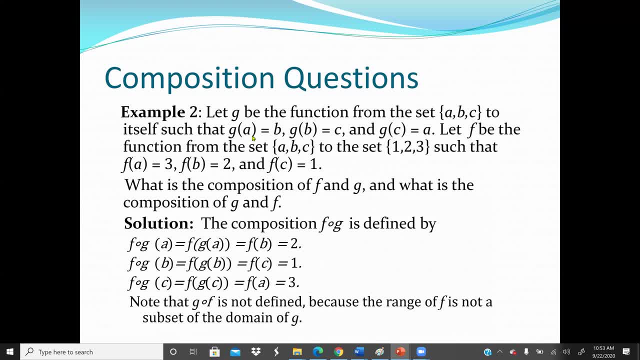 is equal to two, but from the condition we can see that f at b is equal to two. so the next is f composite g at b. so g at b, that will give us f at c, because g at b is equal to c, and that will give us three. 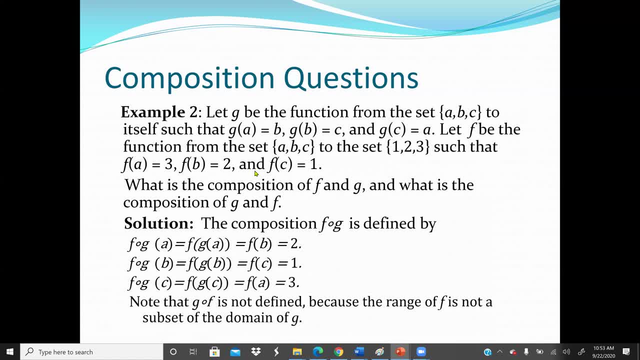 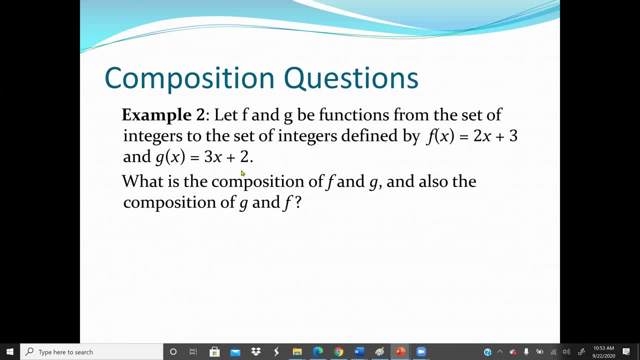 but we cannot find g at f because of the composite, the subset. so another example: let f and g be a function from the set of integers to the set of integers defined by: f at s, equal to 2s plus 3, g at s is 3s plus 2.. 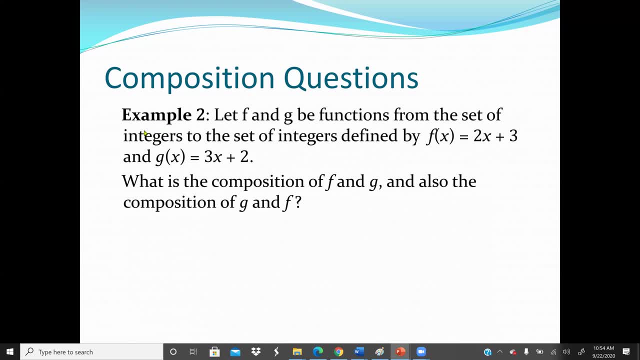 so. so here we have again. second example: f at s is 2s plus 3, g at s is 3s plus 2.. so if i'm finding the composite of f, g at x, first, i'll write down the fx, which is 2s plus 3. 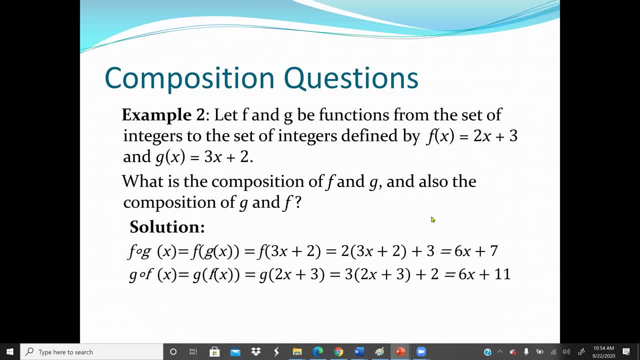 to G at s in X variable. so that's why we get here 2s, for still give. give me 2 times 3s plus 2 plus 3, so againfatace is 2s plus 3, G at s is 3 s plus 2. 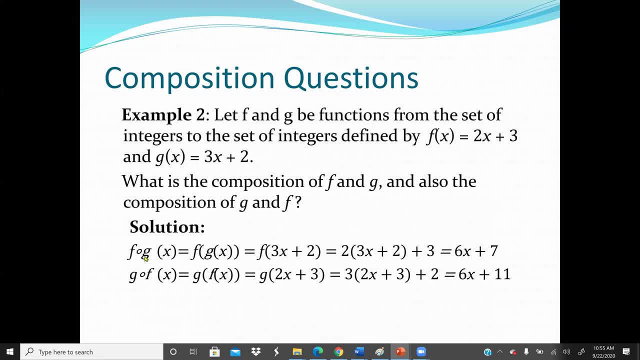 so we get F composite relatx. anyway, once a Gitis, I'm going to substitute with X for FEGった. to find out the term candidate null, I'm just going to substitute with means X for F hat S. thank you so much. I consider some. 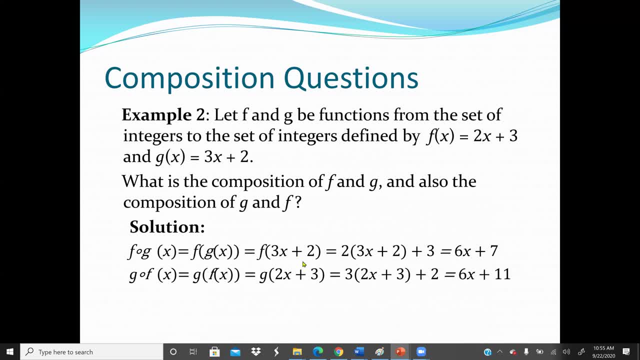 f at x, So we get f at 3 plus 2.. We have 2s plus 3. So s will be replaced by 3s plus 2, because 3s plus 3 is g at s. We find the composite of it, Then we solve it, Then next we find: 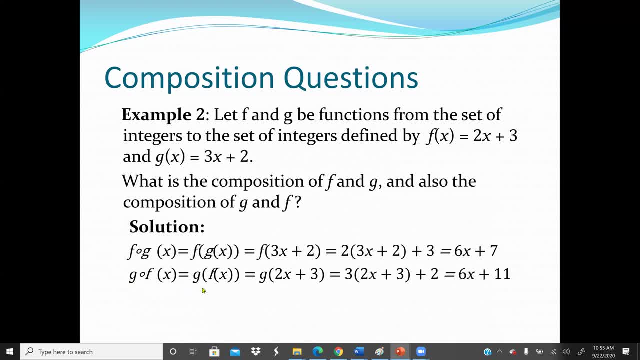 g composite f at x. So we bring g out, We solve the 2f at x in. anywhere we see the variable s in g at x. So we substitute the value here We get 3, 2s plus 3 plus 2.. And then we get: 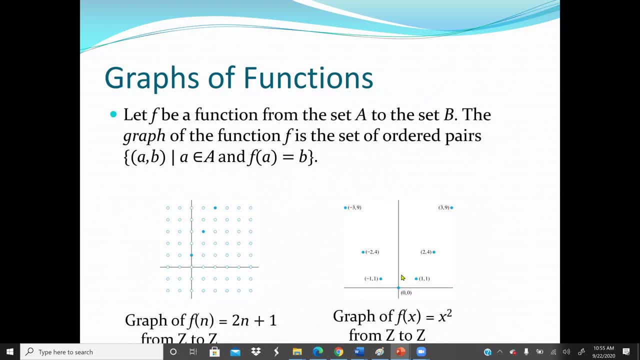 6x plus 11.. So, graphing of a function. normally to graph a function, if it's a linear, if it's a linear graph, we can find the x-intercept. x-intercept is the value of x1, y0.. And then 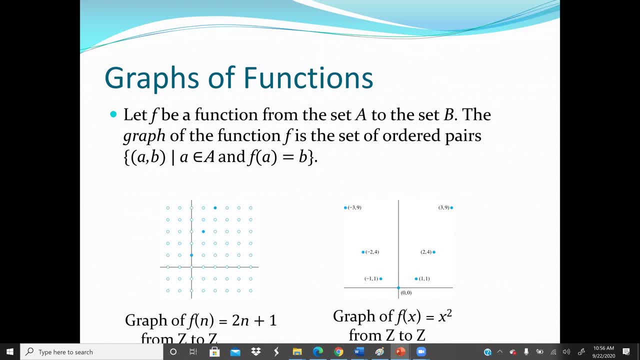 y-intercept is the value of y when s is 0. So when you get the two points then you can draw a straight line across it. But when you are doing it on linear, we need to set a table So we have the input of x, the variable, And we can generate from the function. we. 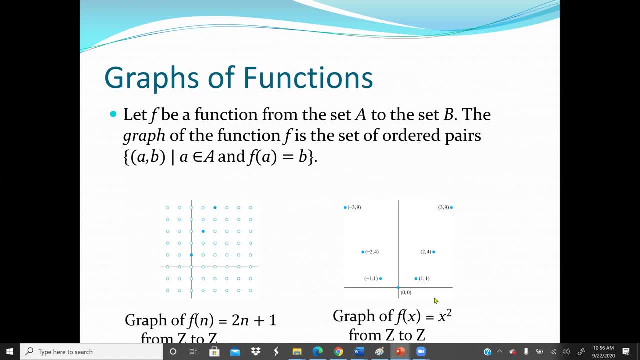 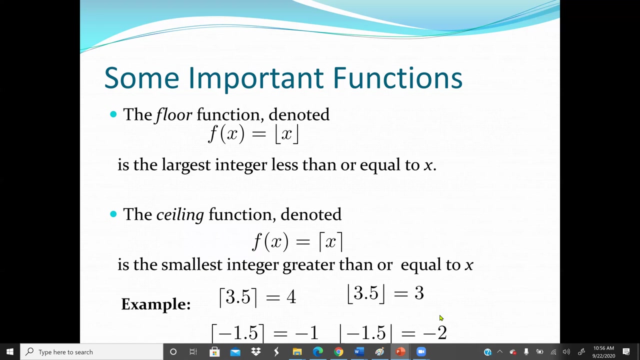 can generate the value of y. So we plot the points, Then we draw a line across the points. So in a linear function our variable exponent is 1.. This is a parabola s squared. Then you're going to get a parabola. 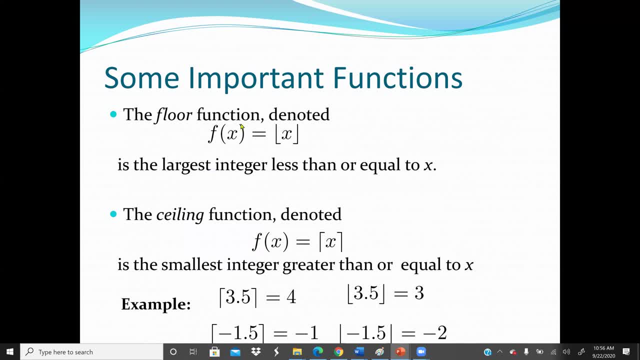 So these are some of the important functions. We have a floor function, which is donated by the symbol here, And it's the largest integer less than or equal to x. The ceiling function also. we have the symbol: It's the smallest integer greater than or. 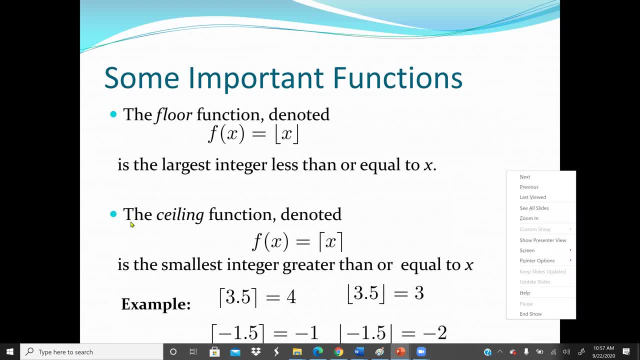 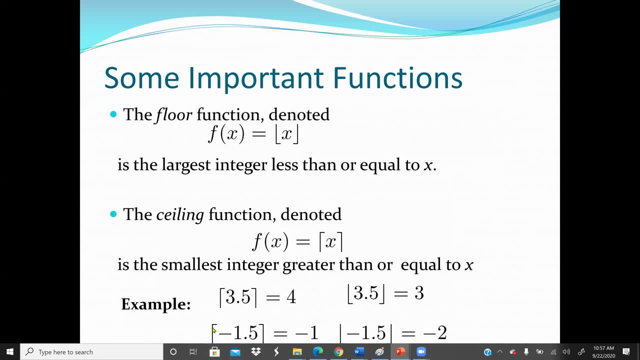 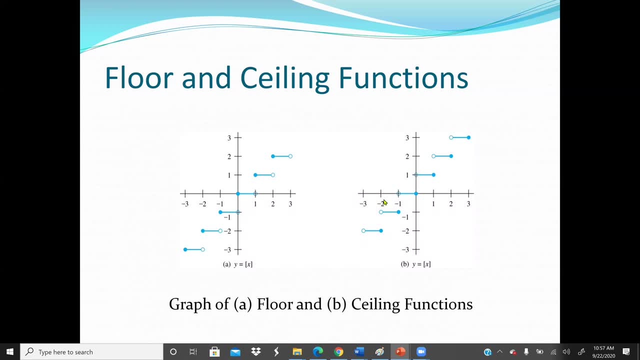 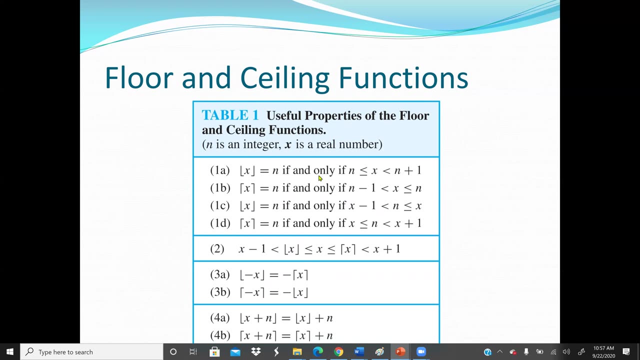 3.5.. The ceiling will give me negative 1.. So that's our floor and ceiling functions And these are some of the useful properties of the floor and ceiling functions. So when we have the first, which said it means s is less than or equal to n and greater than n. 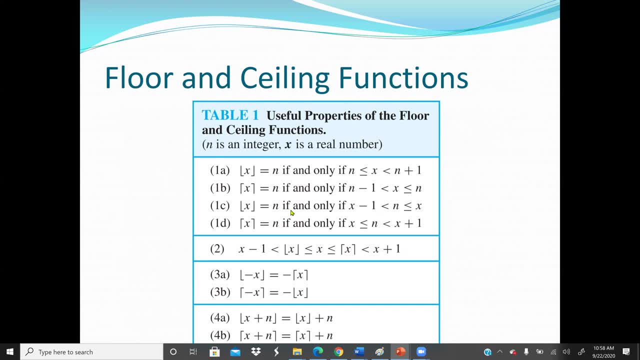 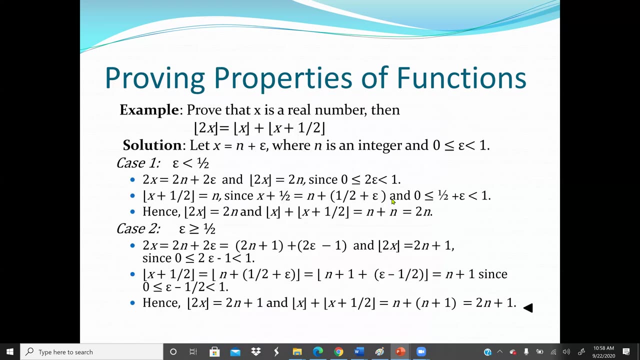 plus one, And then it's also the same n minus one. s is less than n minus one and less than equal to s. also, We can also prove the properties of a function. For example, prove that s is a real number, then we have this. I want to prove this as a real number. We may have two. 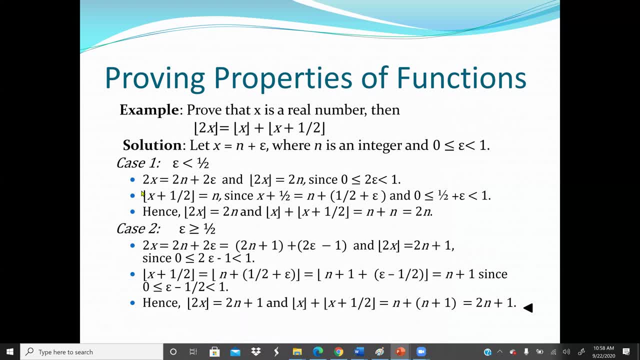 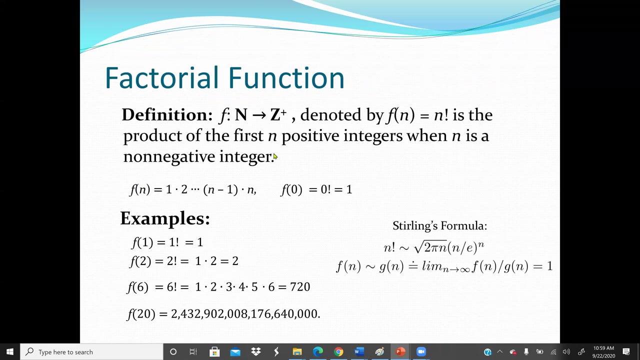 cases. One case is: if the decimal value is less than 0.5, then we ignore it. The decimal value is greater than or equal to 0.5, then we approximate it to one, And that's the step here. The factorial of a function, again, is a function that we multiply. 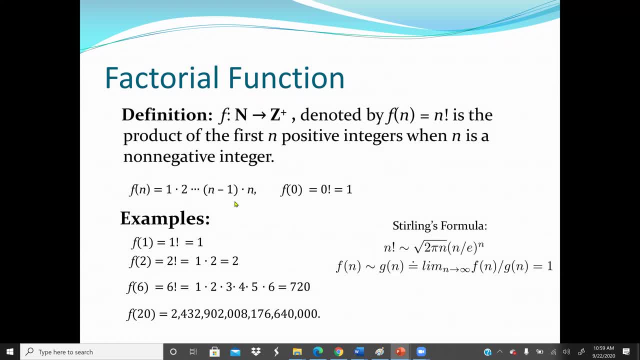 If we are looking for a factorial of five, they need to be five times four times three times two times one. We say that a factorial of a function is donated by F. at n, the work is n, Then exclamation is the product of the first n positive integer when n is non-negative. 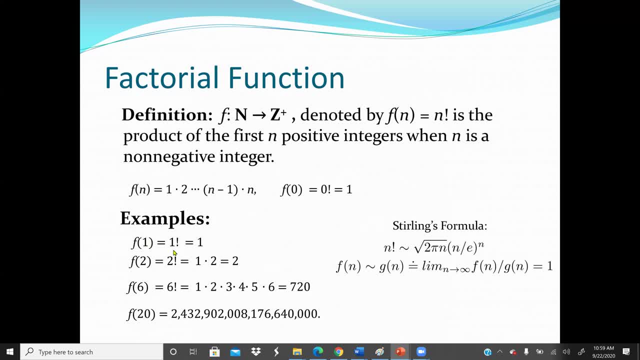 integer. So we may have F at a, sorry, F at one. the factorial of one is one, factorial of two to be two, Then factorial of six will be one. One times two times three times four times, five times six. Factorial of two will give me one times two. 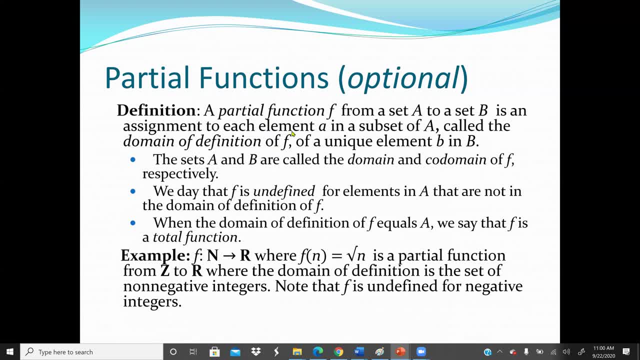 We also have what we call the partial functions. Here we say a partial function F from a set A to set B is an assignment to each element A in a subset of A called the domain of the function of a unique element B. So a set of A and B are called the domain and codomain of F respectively. 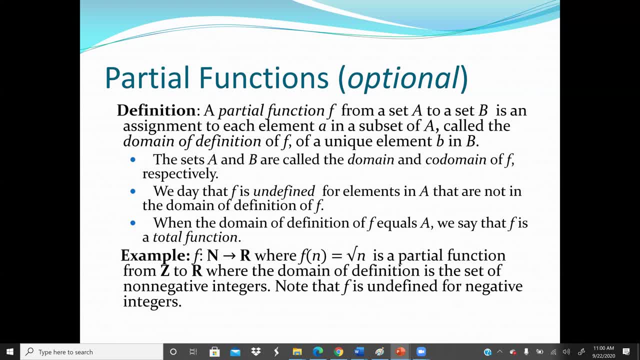 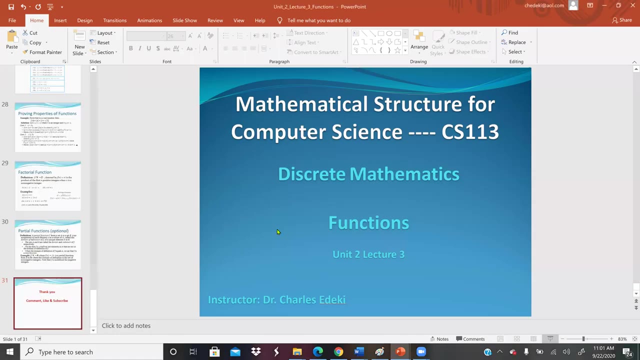 Also we can say that F is undefined for elements in A that are not in the domain of a definition of B. So when the domain of a definition of F equals to A, we say that F is again a total function. So this will be the conclusion of, again, session 2.3..